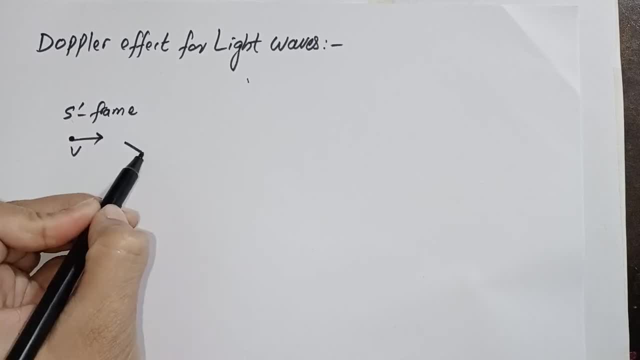 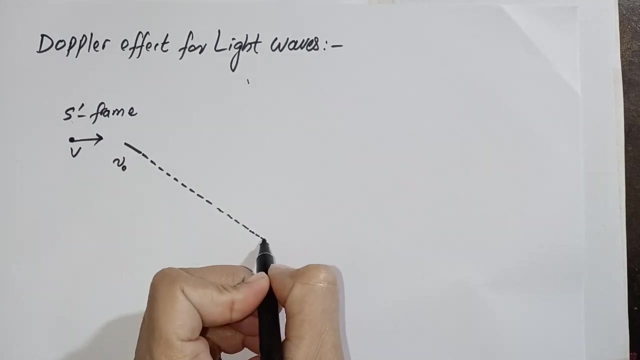 is Z 1, which is theae on the N FR amount V 0.. Phoenix, which is the voltage of ring Time, Z to nK, as C, 0 pixels to st. energy emitting a light signal with frequency proper, frequency nu not. this signal will approach to stationary observer in rest. 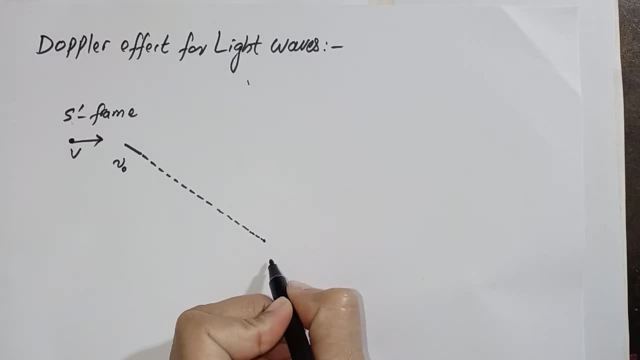 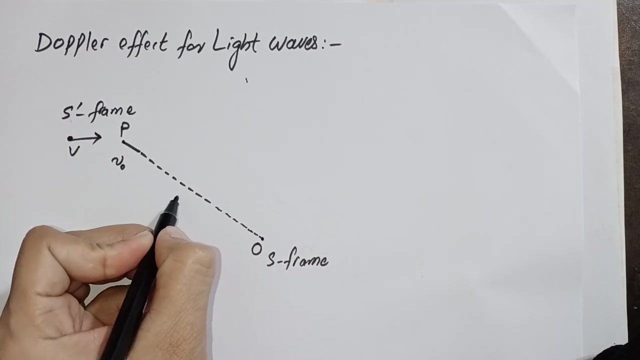 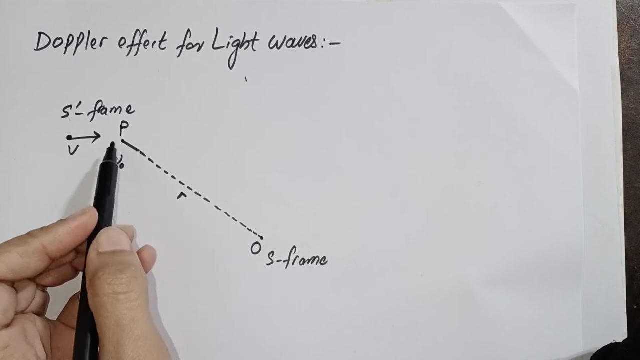 frame of reference and this point, we have a rest frame. the signal is emitted at point B and it is received at point O by stationary observer. it will cover a linear distance, R, and the time taken for the light signal to reach at point O will be according to. 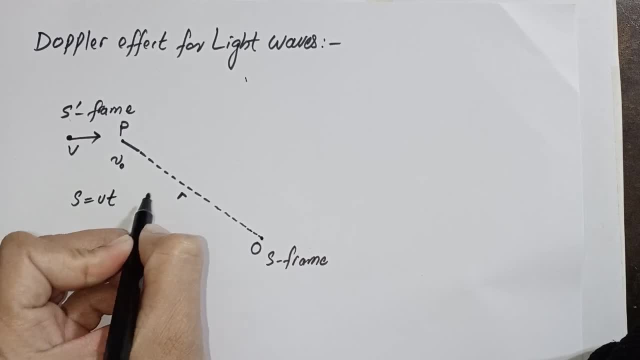 linear equation s equal to Vt. distance covered is R, then the time taken will be R over V, since it is a light signal, so this V will be replaced with C speed of light. the time taken to reach this signal, which is emitted at point B to point O, will be R over C. 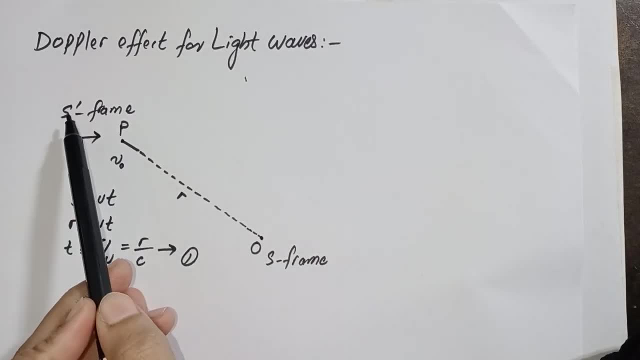 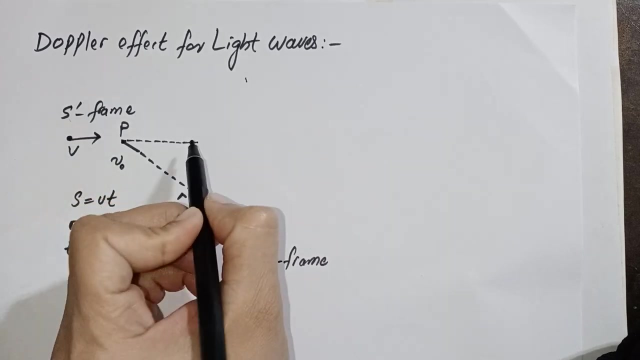 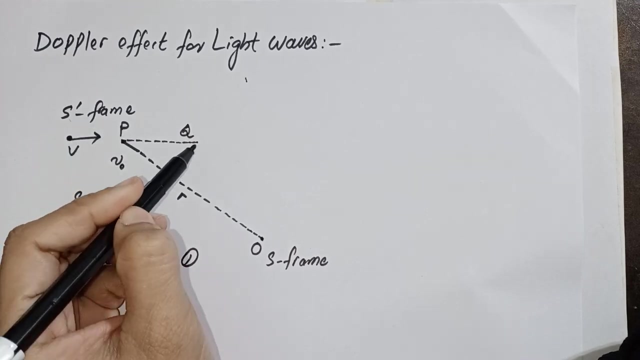 since this source is moving along with S prime frame. so when the signal is received at point P by this rest observer, it will move to next position, let's say at point Q, and then it will again emit a light signal at this point Q and this rest observer will receive it at this point. 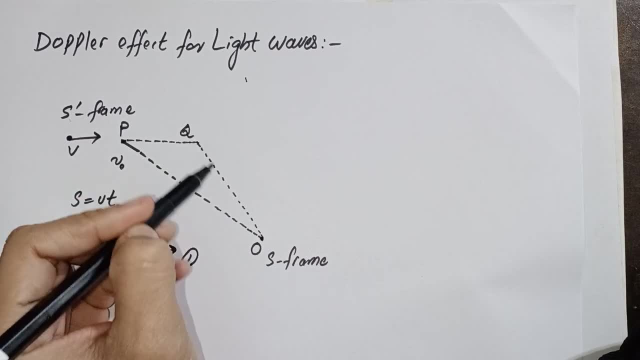 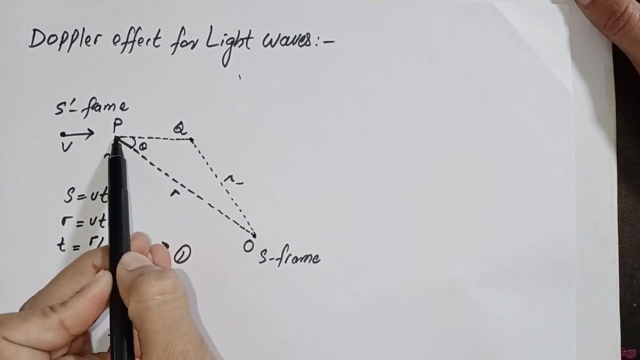 for next stop response and then it will move to next position. and then it will. it will- let's say it will- cover a distance- R prime- from Q to O, and t0 will be the time taken for the source to move from this point towards point Q. then this linear distance will be vt0 and and we can draw a. 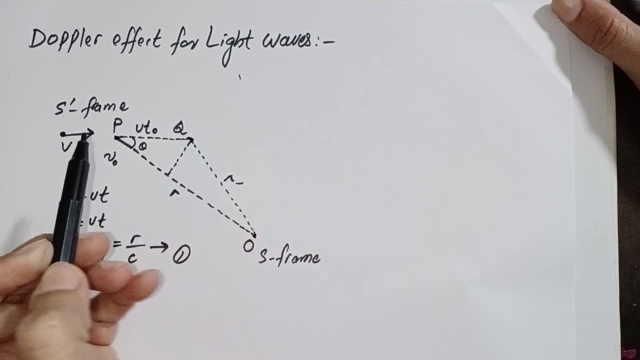 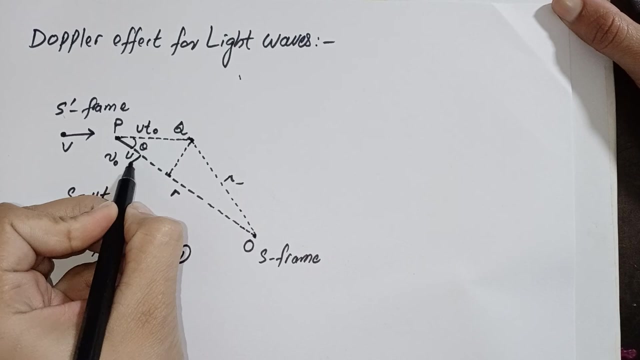 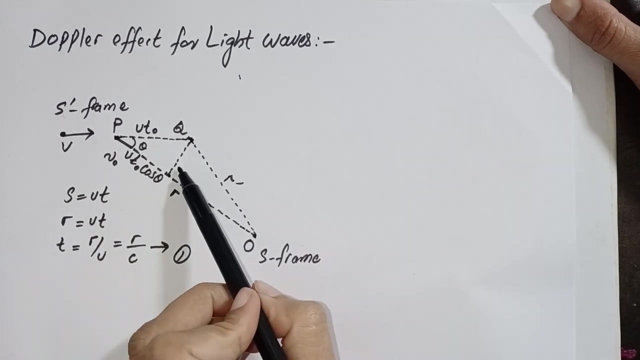 perpendicular from this point and can supplte this geometry into two components. this will be the vertical component, this will be the horizontal component. this horizontal component will be B 10 cos of theta, and vertical component will be VT naught sine of theta, since we only need this. horizontal component. we can just hand Mortal Cos of theta, zł z0hearted of theta and som pissed from the lower testет 0 to z0 here. the horizontal component here isブ of θPl seguirъ 날 because of theta, and vertical component will be B t0 sine of theta, since we only need thispolit zwe audienceرة. that is therefore now we can see the. 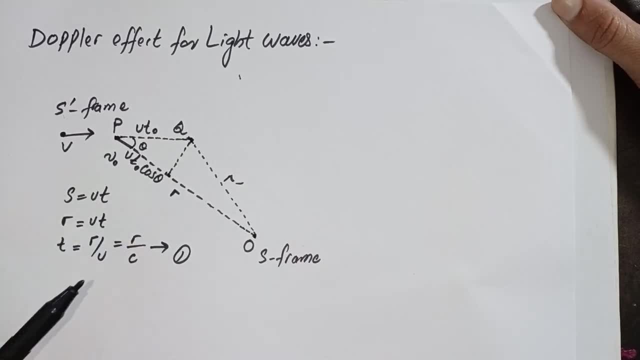 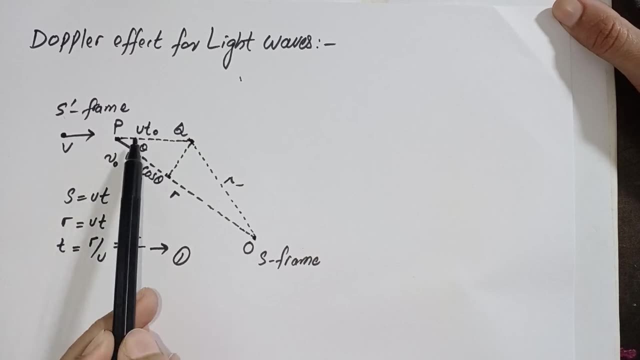 component. so we will not label this vertical component for simplicity. in the time taken for this second signal to reach at point O will be the time taken to move this source from P to Q and the time taken to reach this signal from Q to O. so since this time is t0 for this distance, this time is t0, then it will be. 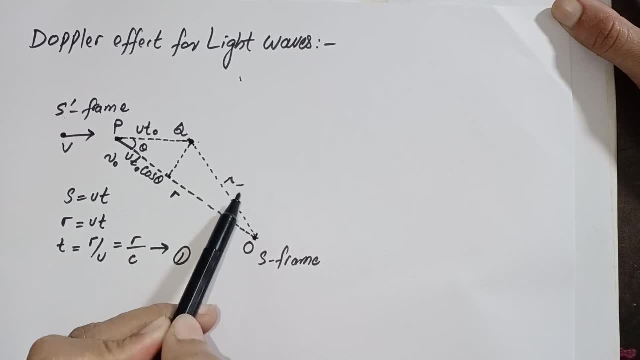 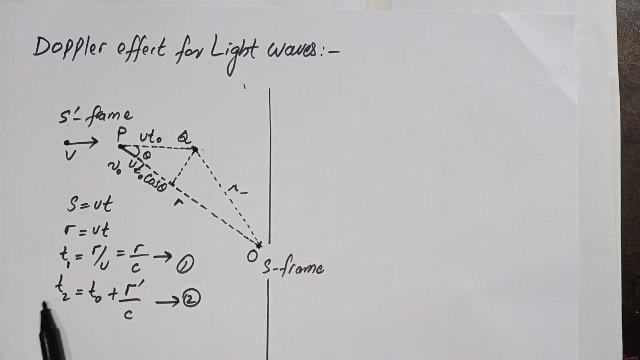 t0 plus this distance, which will be R prime over C, so that we define this with t1, then t2, which will be the time to reach the signal, to reach the second signal at point O, it will be t0 plus R prime over C, then the time difference between these two light. 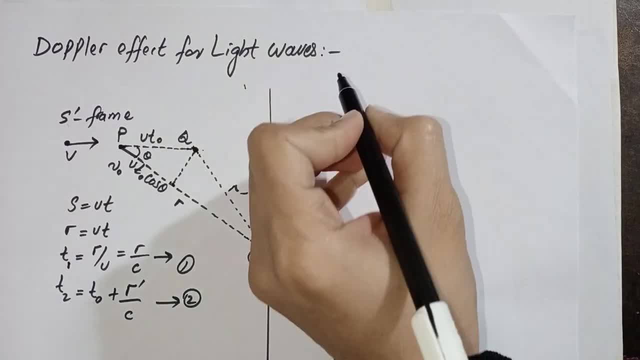 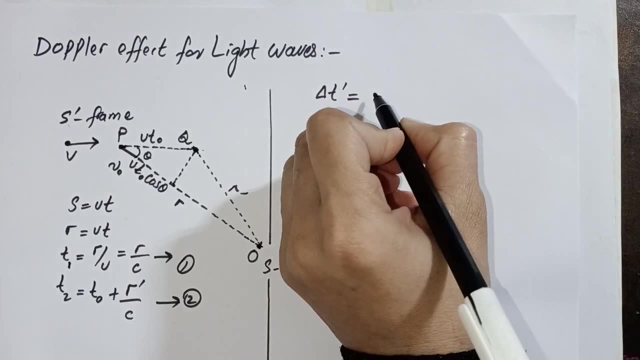 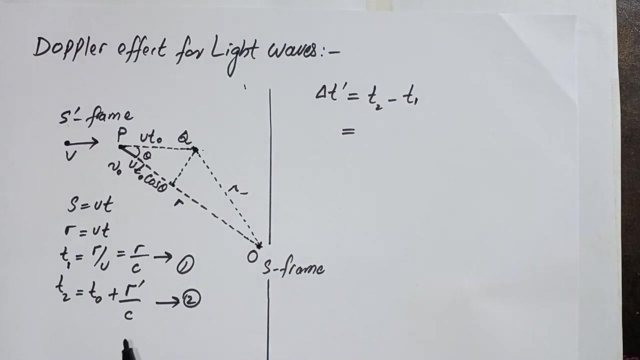 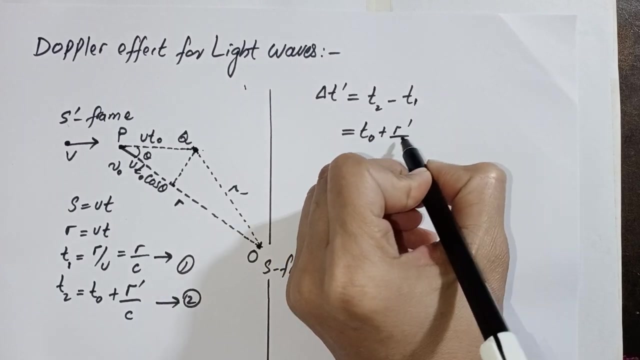 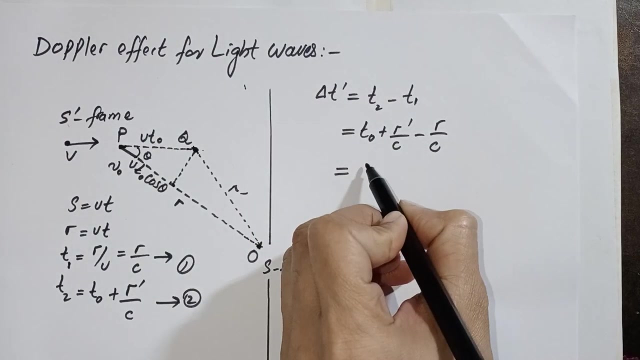 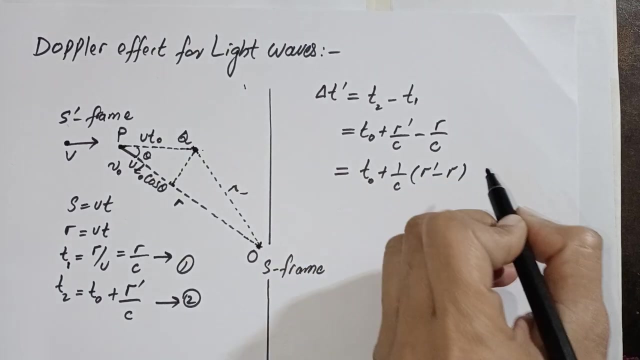 signals to reach at point O will be, let's say, the time difference is delta, t prime, it will be t2 minus p1. substituting the values, t2 is t0 plus R prime over C minus t1 is R over C will be t0 plus 1 over C, R prime minus R. now we will find out the. 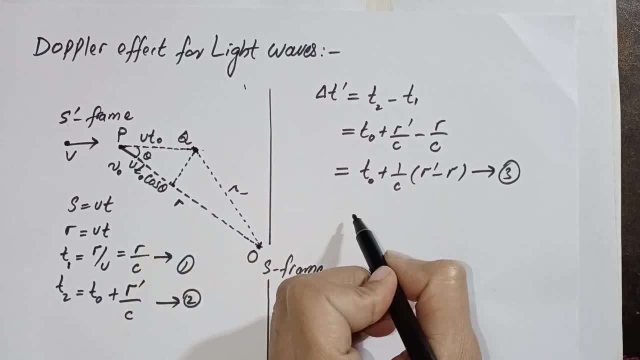 value of this R prime. from this diagram we can see that this r prime is this length. r prime is this: total length is r r minus this component, v t naught cos of theta. it will gives the value of this r prime, so it will be r minus v t naught cos of theta. substituting in equation three, we will have delta t prime. 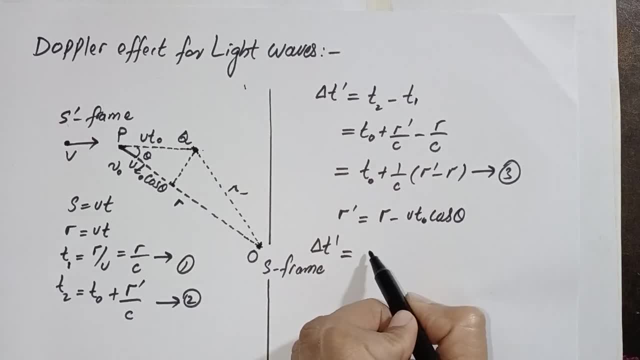 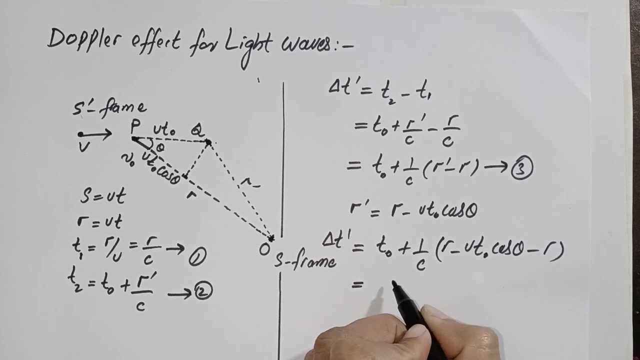 equals to t naught plus 1 over c. this r prime is r minus v t naught cos of theta minus minus r, and it will be t naught into 1 minus v t naught over c cos of theta. now we will define this ratio. 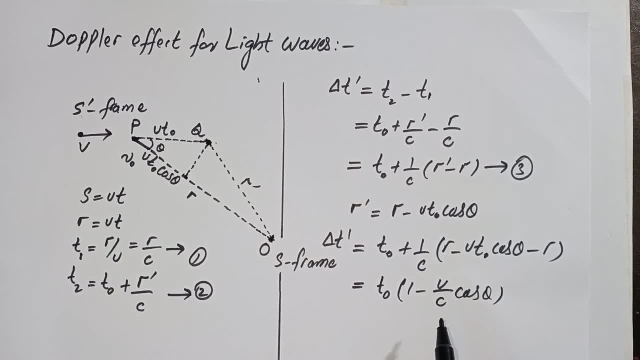 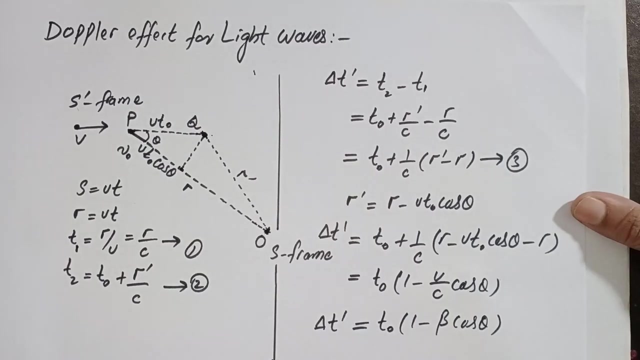 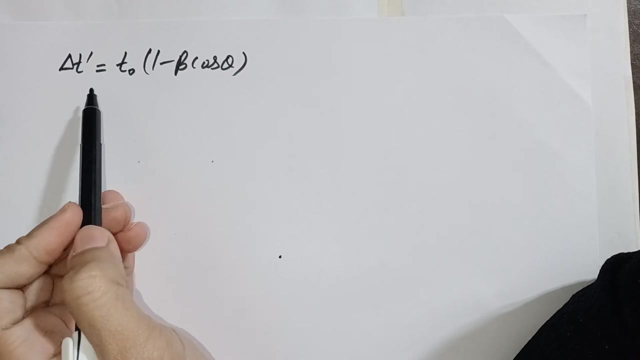 ratio of speeds with beta. so replacing v over c with beta, then delta t prime will be t naught into 1 minus beta cos of theta. this is the time difference between the two light signal to reach at point o after reaching the point of o. so this delta t prime. 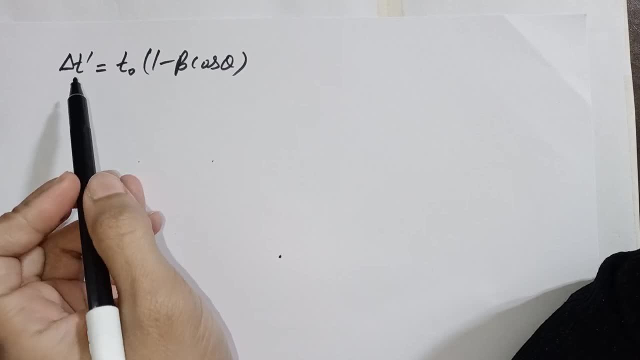 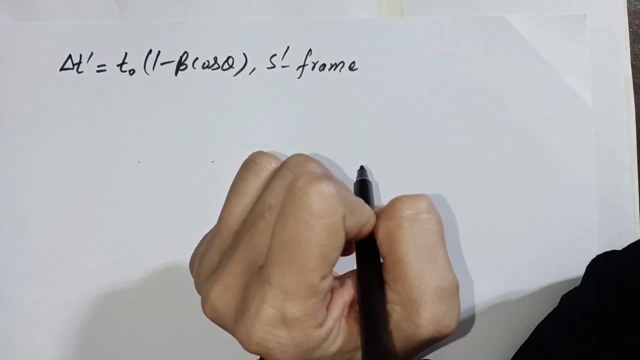 is the time according to s prime frame. is the time. is the time according to moving frame of reference. according to s prime frame of reference. according to moving frame of reference: is the time. Similarly, we can write the time difference for the two light signals according to rest. 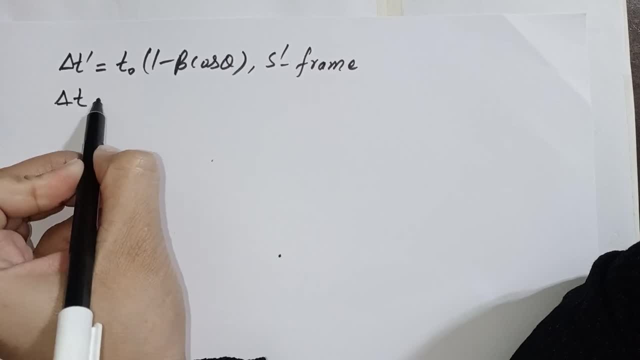 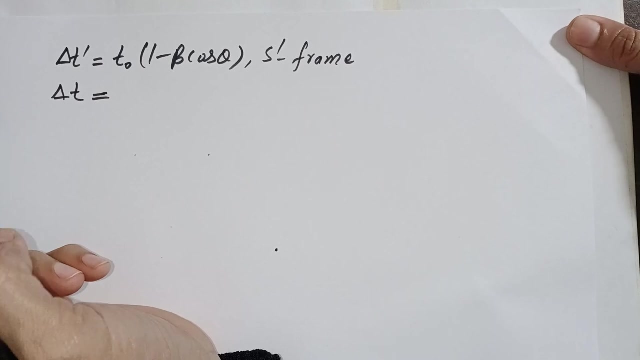 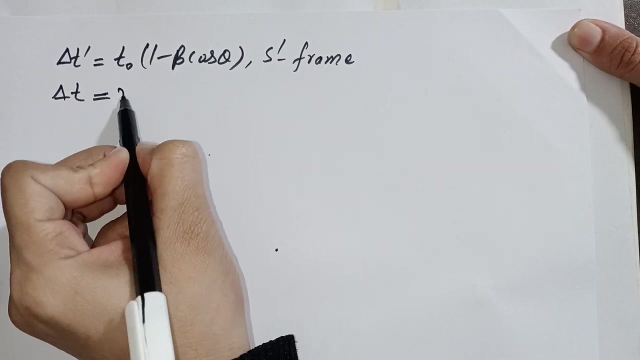 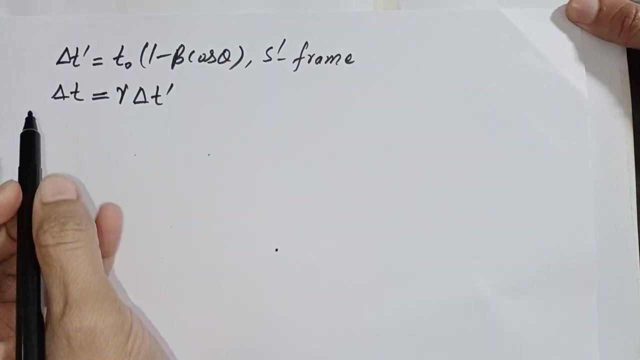 frame of reference, which will be delta t prime, is for moving frame of reference, then this delta t will be connected with this delta t prime according to time dilation principle. this delta t will be gamma times delta t prime. We will use the concept of time dilation to link the time difference between the two light. 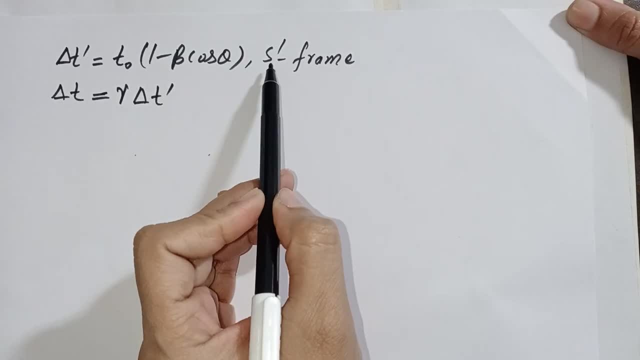 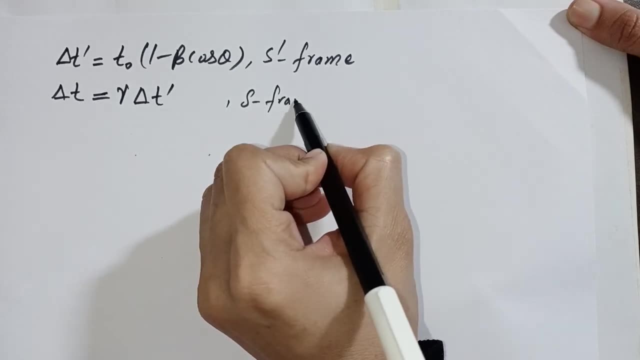 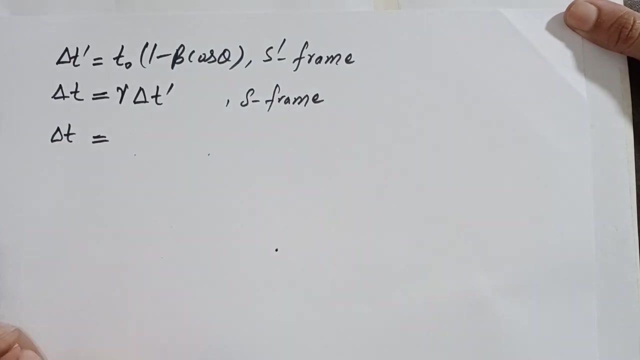 signals. So this is as observed by moving observer and as observed by rest observer in frame s. So, substituting the value of delta t, prime delta t will be gamma p. nor into 1 minus beta cos of theta. Okay, Okay. 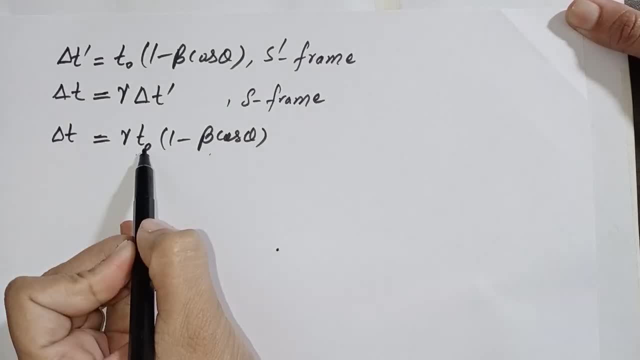 Now we will relate this time t with frequency of light signal. this is: the light signal was emitted at proper frequency nu naught. then this t? naught will be linked with the nu naught, which is inversely proportional. nu naught will be 1 over t naught and then nu will be. 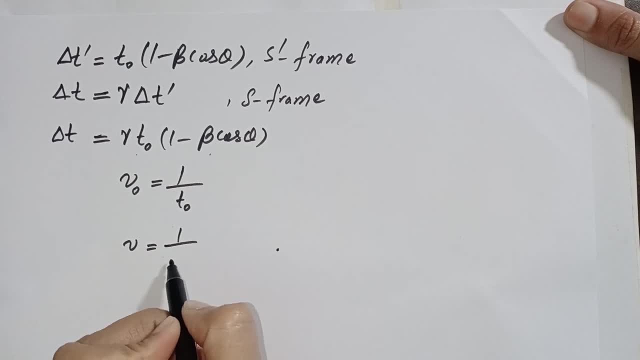 frequency. Okay, Okay, Great So. so for the time being, little time will be 1 over t, or we can write it as 1 over delta t, Since we are measuring the time difference between two light signals. then this frequency: 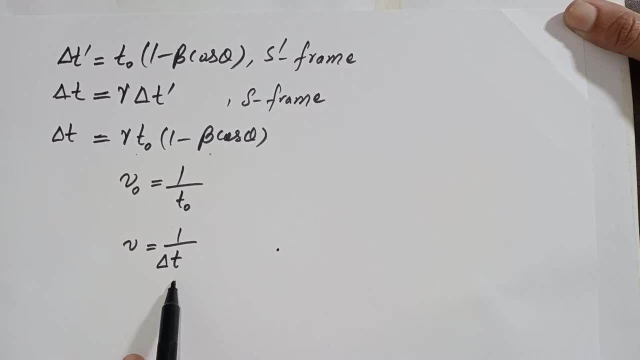 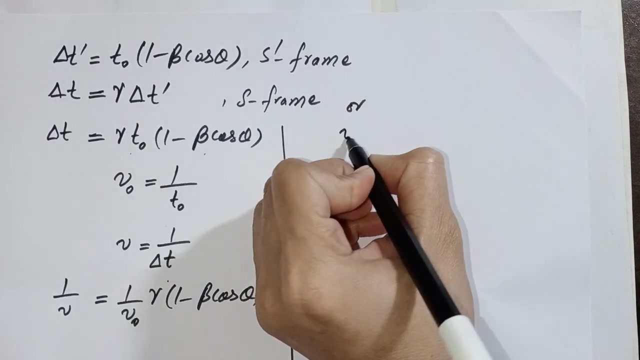 will depend on this time difference, delta t. So replacing delta t with 1 over nu, Okay Okay. and t0 with 1 over nu0, the expression will be: 1 over nu equals to 1 over nu0 into gamma, into 1 minus beta cos of theta. or we can write: nu equals to nu0 over gamma. 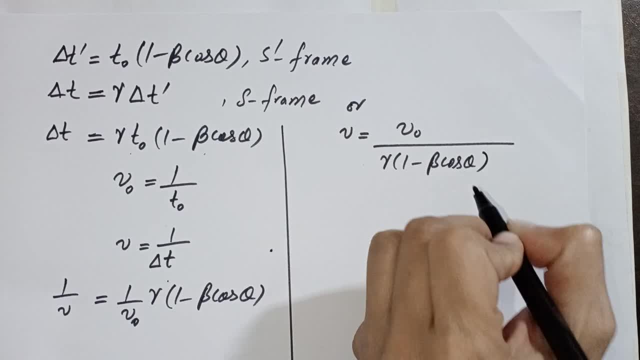 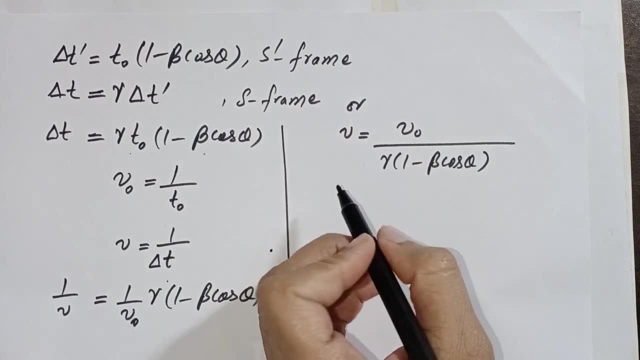 into 1 minus beta cos of theta. We can also relate this expression, This frequency, with wavelength of light signal by using formula c equals to nu0, then this expression will be lambda- equals to lambda0 gamma. into 1 minus beta cos of theta, which. 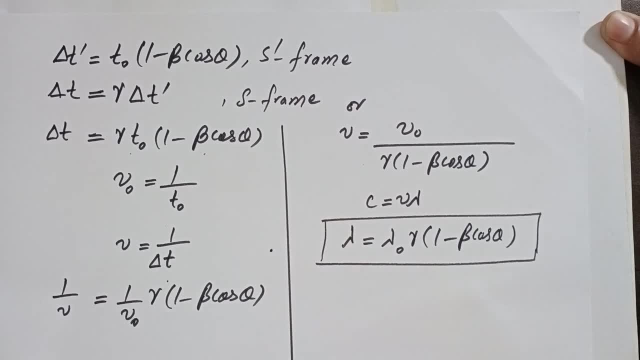 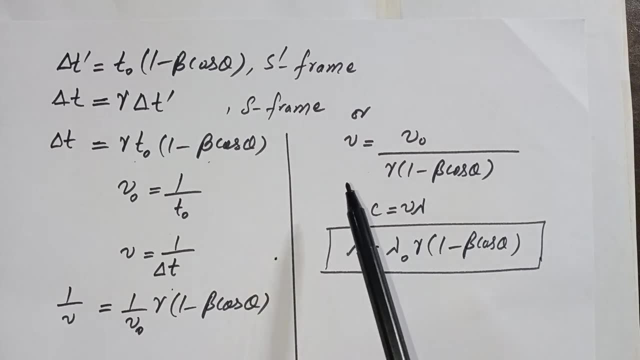 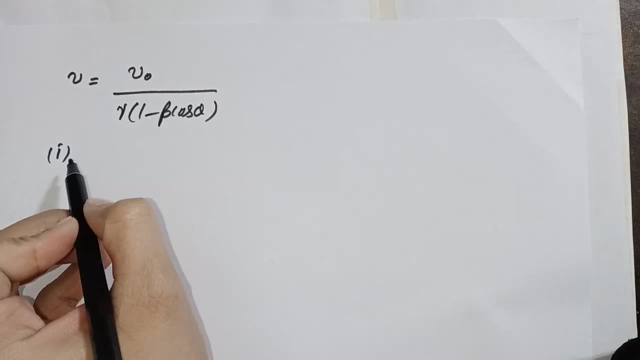 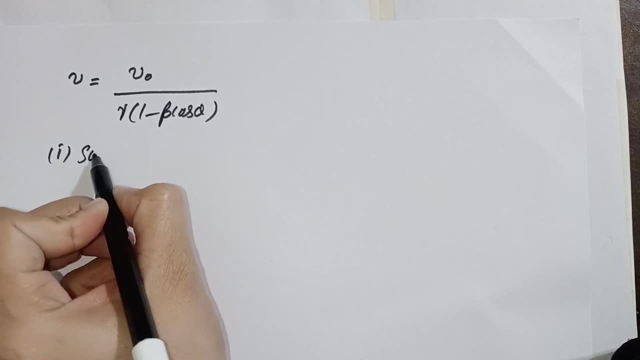 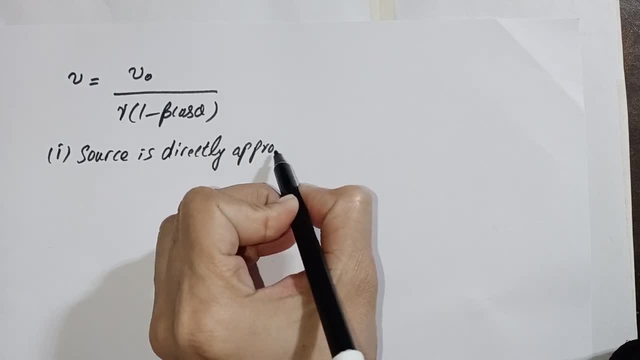 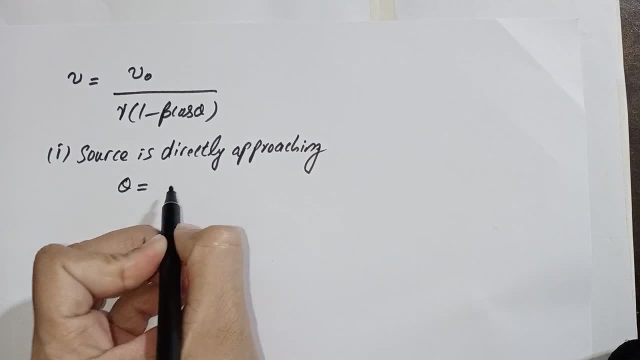 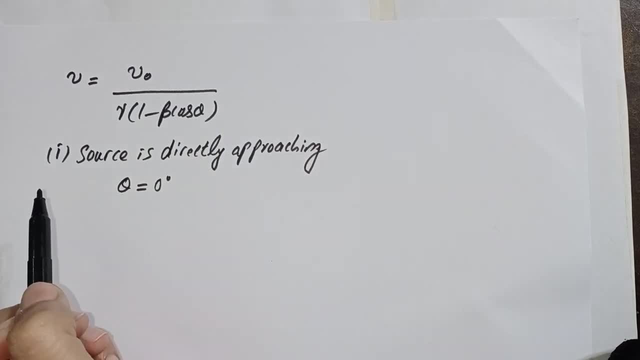 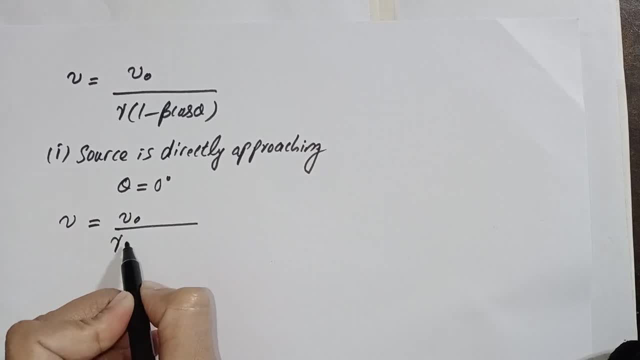 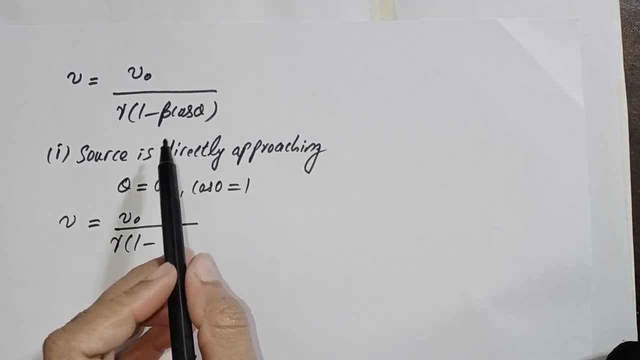 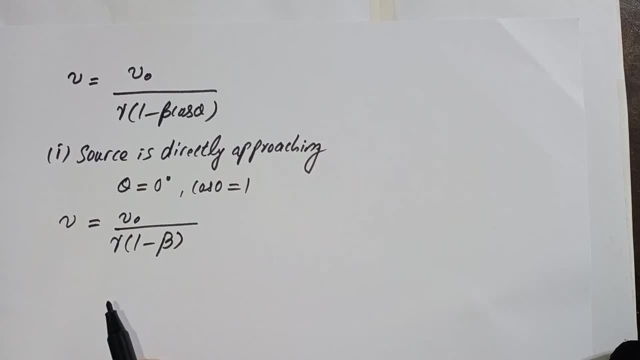 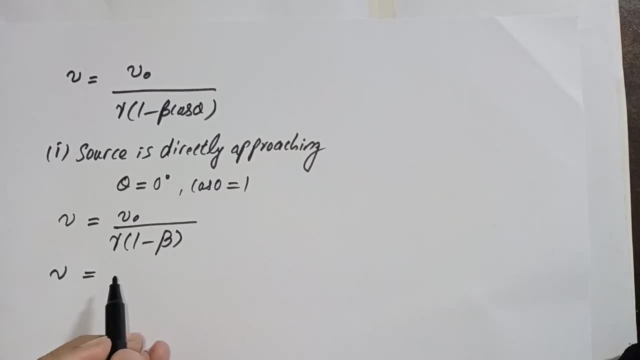 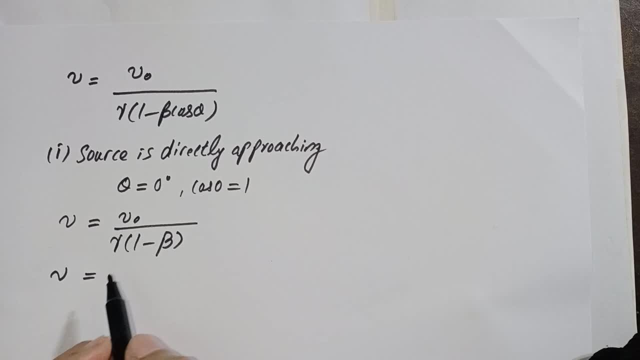 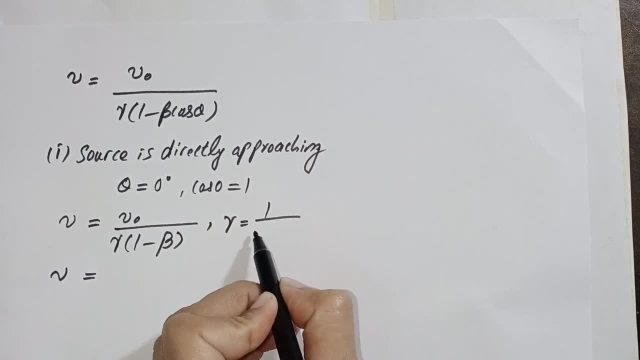 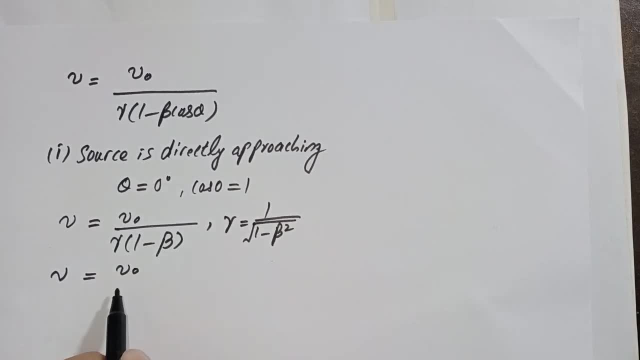 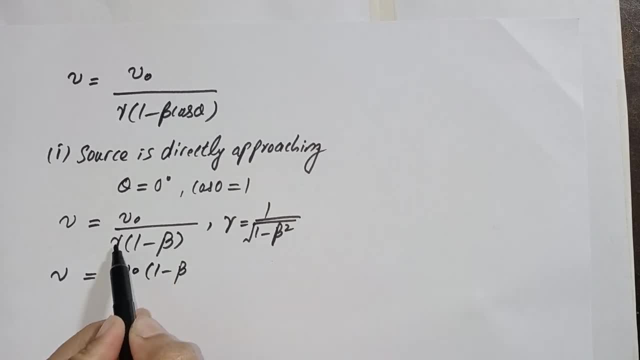 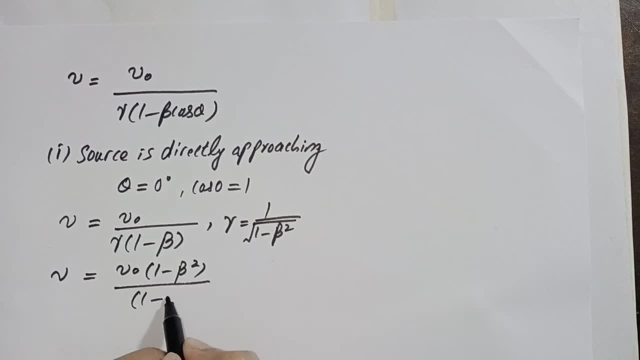 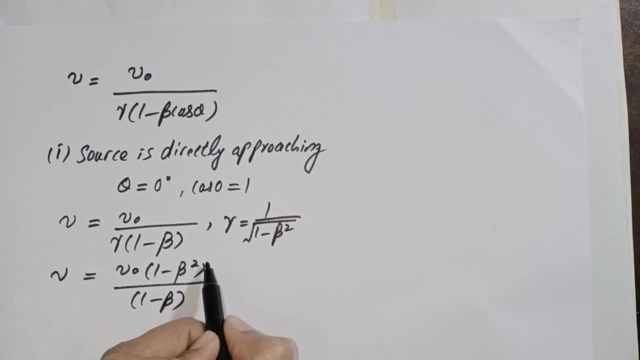 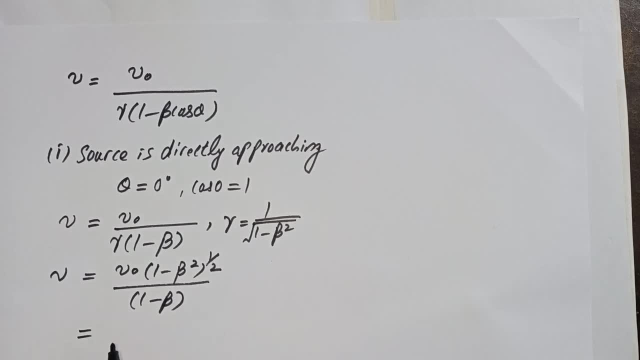 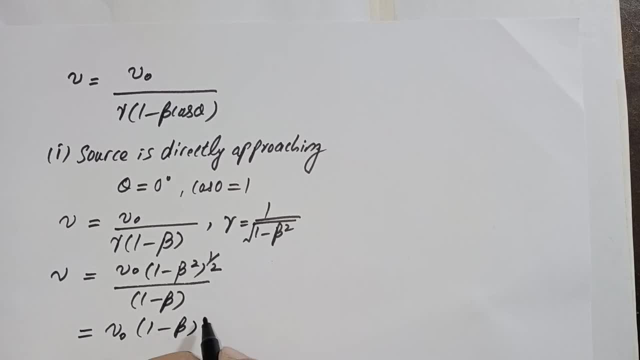 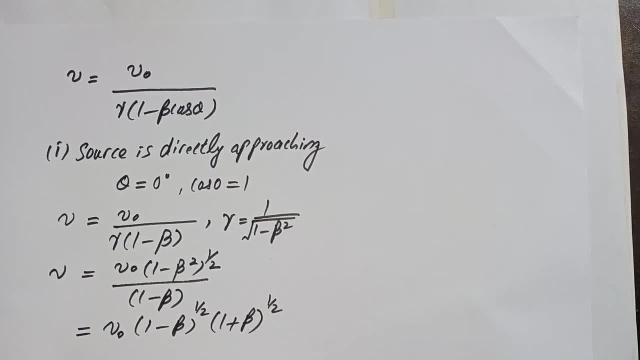 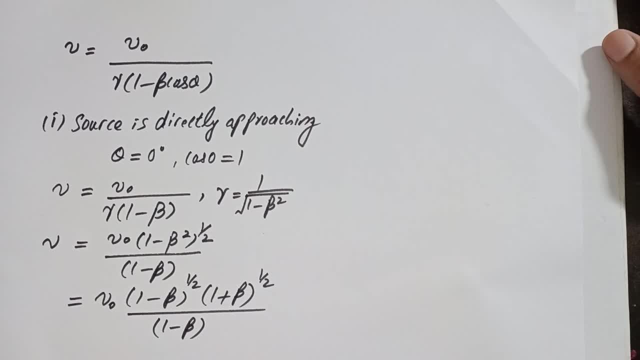 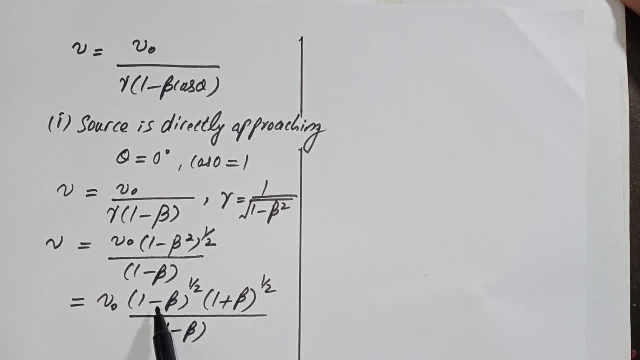 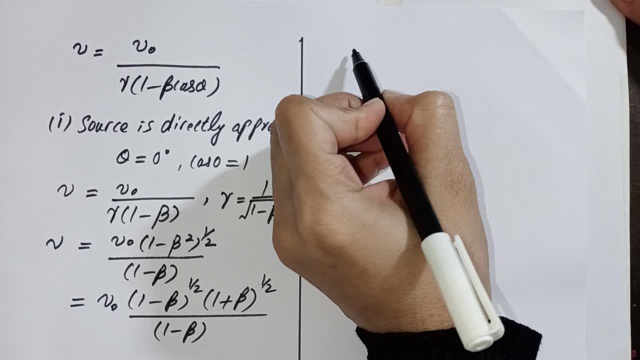 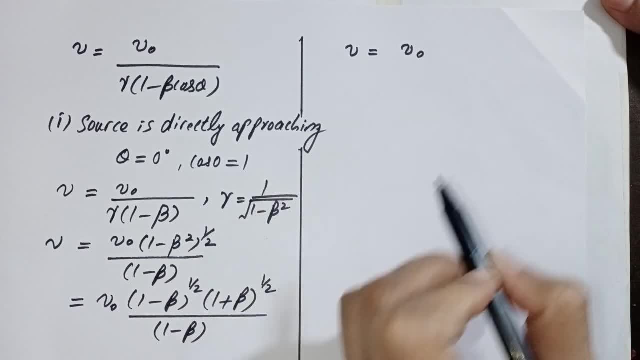 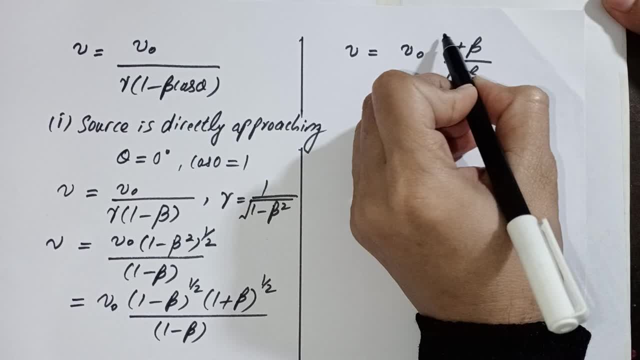 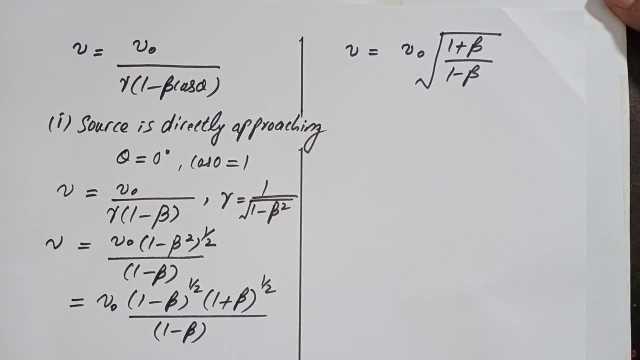 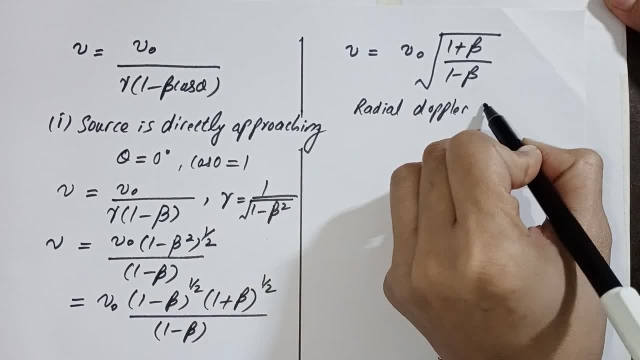 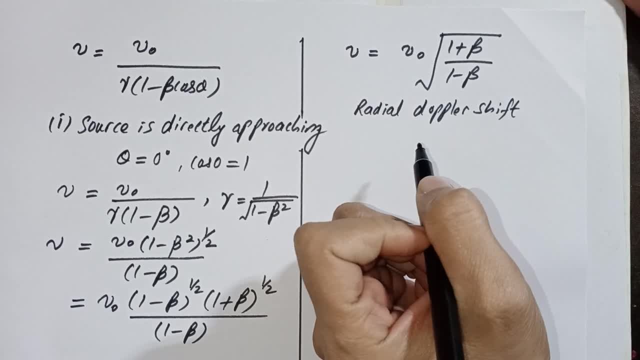 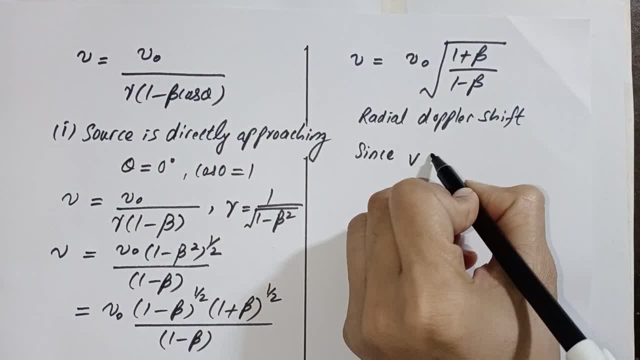 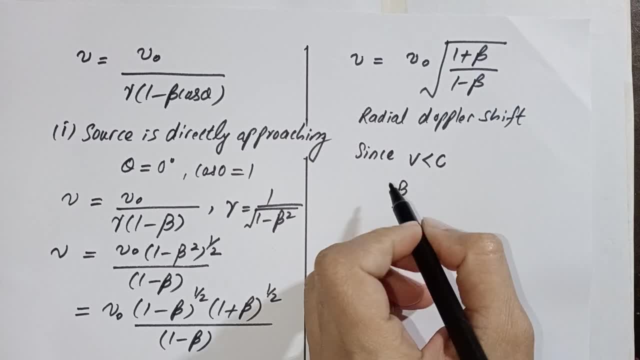 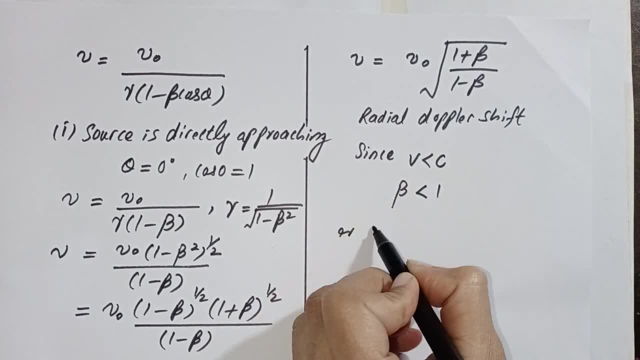 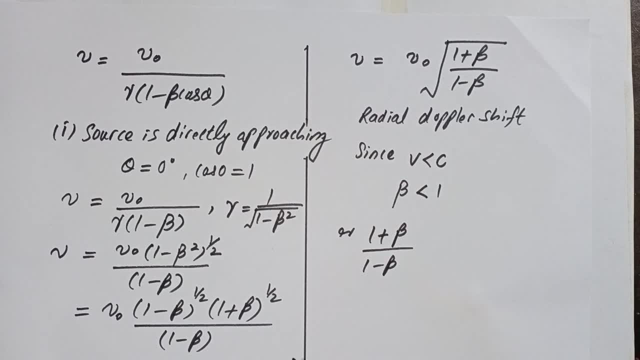 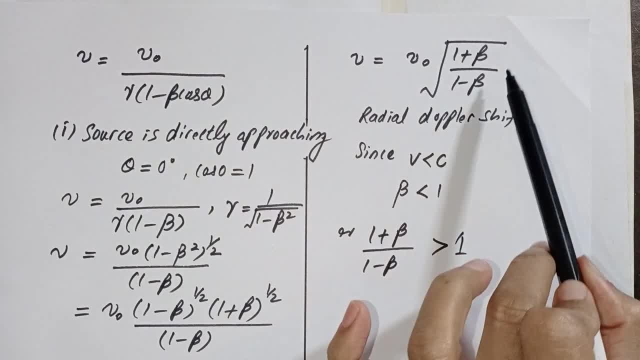 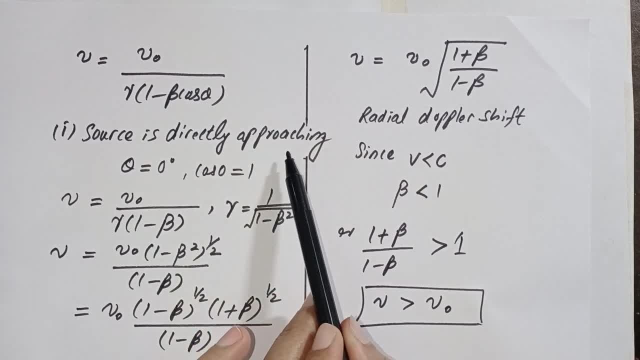 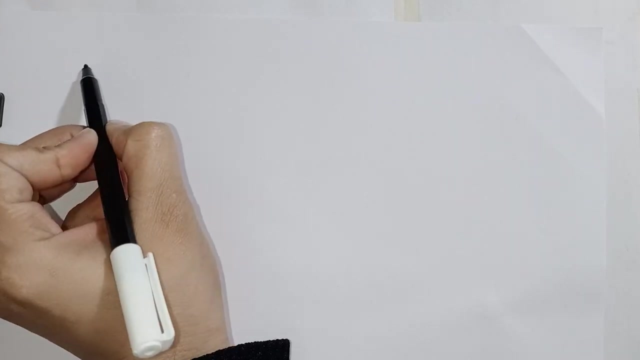 frequency if the source is directly approaching towards stationary observer. next we will discuss a case if the source is receding directly from the observer- like the source is moving away from observer- then what will be the shift in frequency? if the source is moving away, it means theta will be 180. so if the source is moving away from observer, then theta 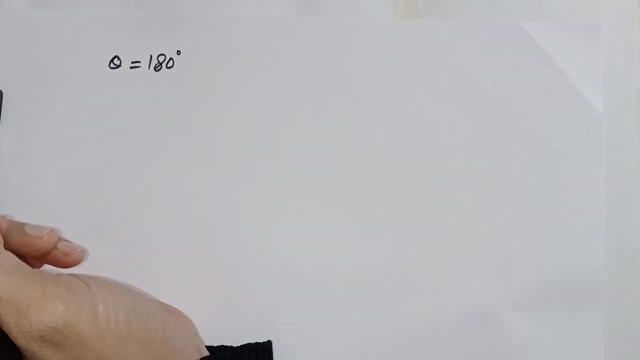 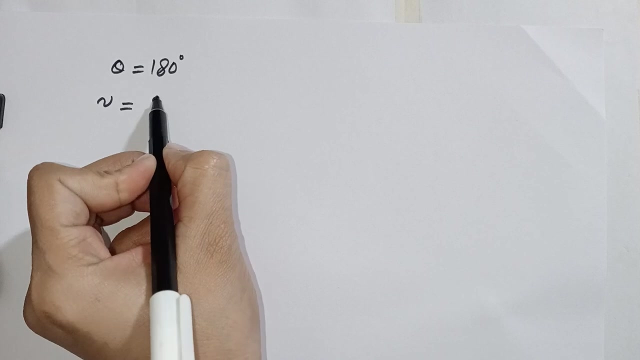 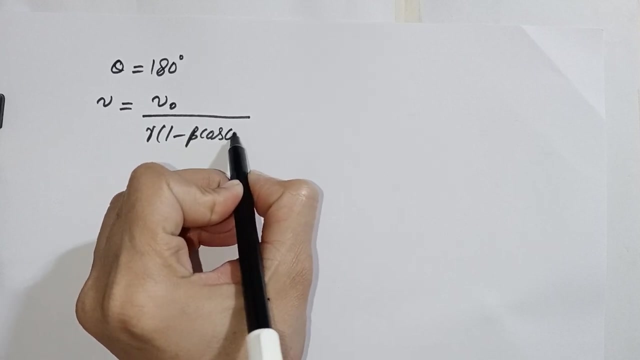 will be 180 degrees, again using the formula for Doppler shift in frequency, given to be 180. so if the source is receding away from observer, and irrespective of how, which is nu equals to nu, not over gamma, into 1 minus beta, cos of theta, cos 1, it will be minus 1. 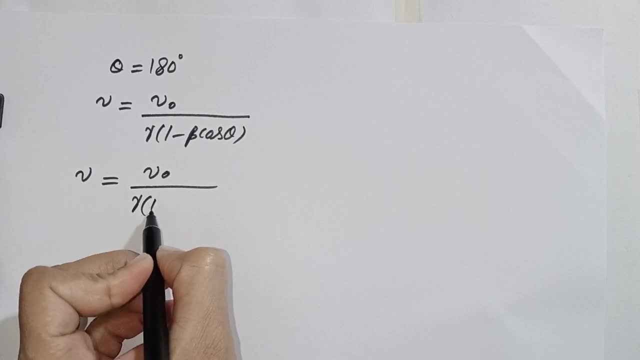 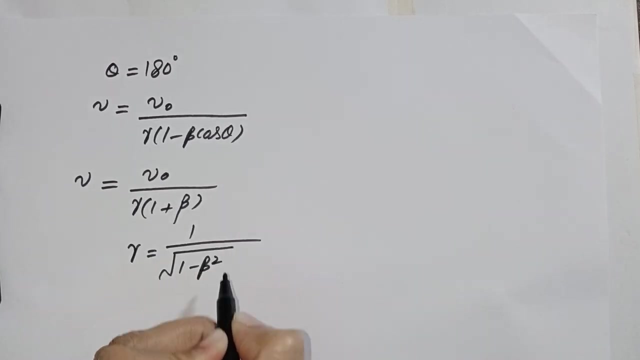 and nu will be nu not over gamma, into 1 minus cos 1, it is minus 1, then it will be 1 plus beta, Substituting the value of value of gamma, which is 1 over 1 minus beta square. 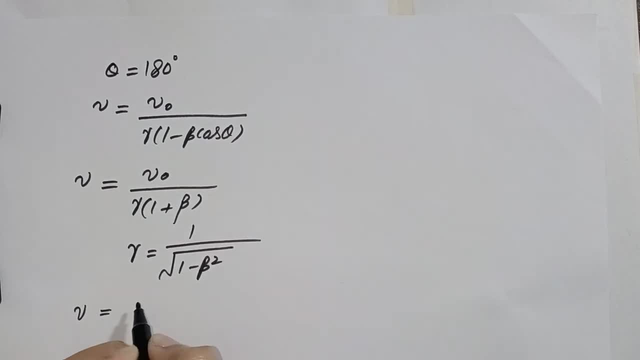 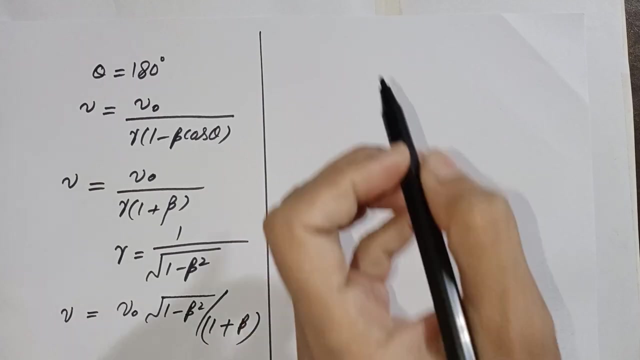 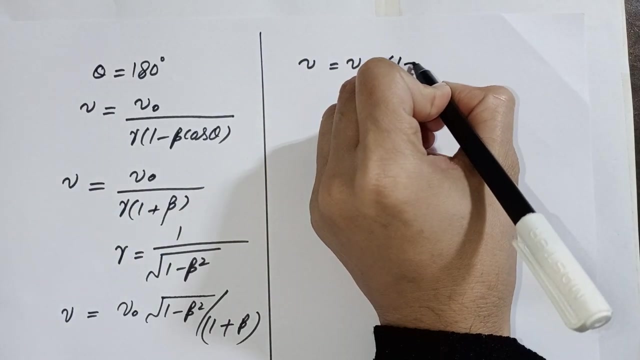 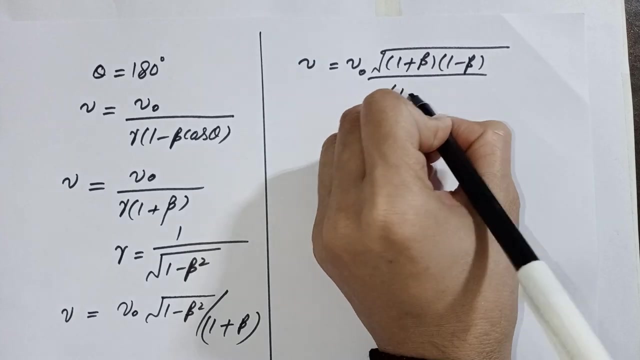 So it will be nu not into 1 minus beta square. So it will be nu not into 1 minus beta square over 1 plus beta. Again, splitting this term 1 minus beta square nu equals to nu not 1 plus beta- into 1 minus beta over 1 plus beta. 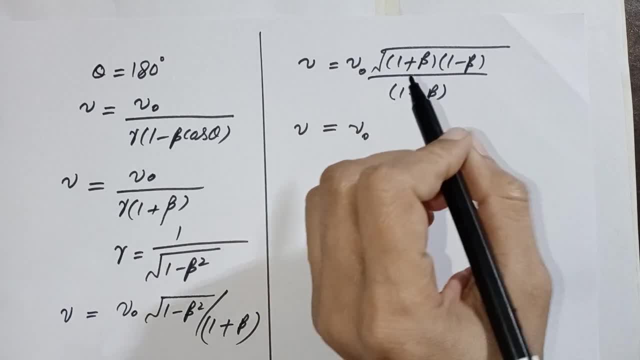 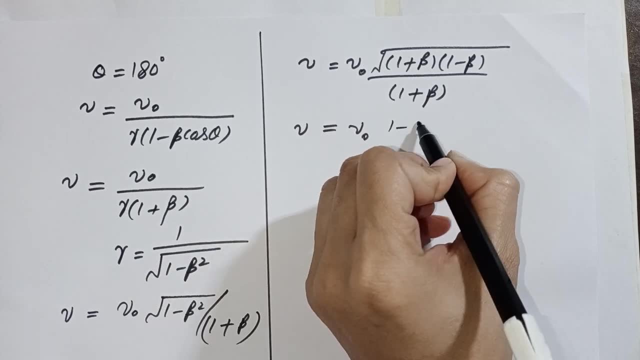 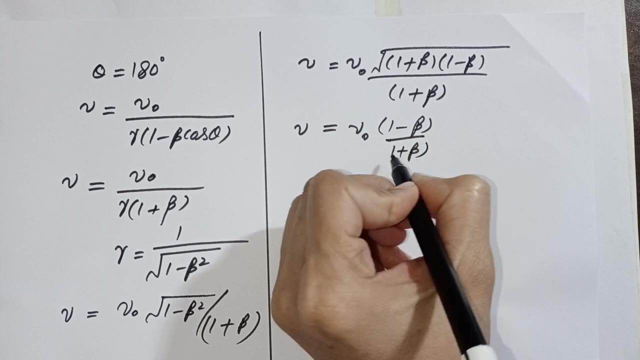 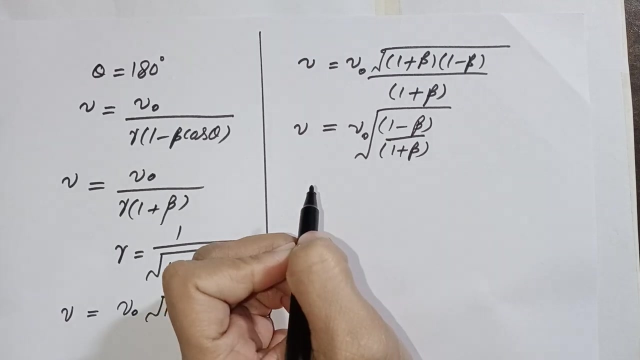 It will be nu, not This: 1 plus beta will be 1 minus beta over 1 plus beta, whole square root. So this will be the shift in frequency If the source directly decedes from the source, Now observer. Now we will again discuss the case. 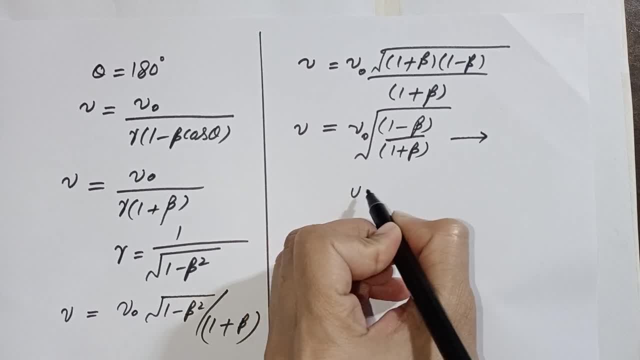 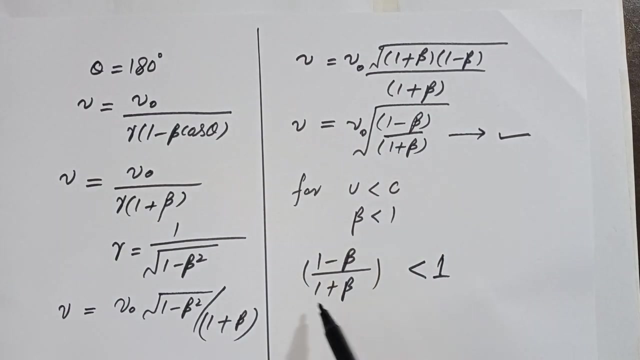 That is, for v smaller than c, beta is less than 1.. And this ratio 1 minus beta over 1 plus beta. So for beta less than 1.. This ratio will be less than 1.. According to this formula, if this ratio is smaller than 1, then nu will be smaller than nu, not. 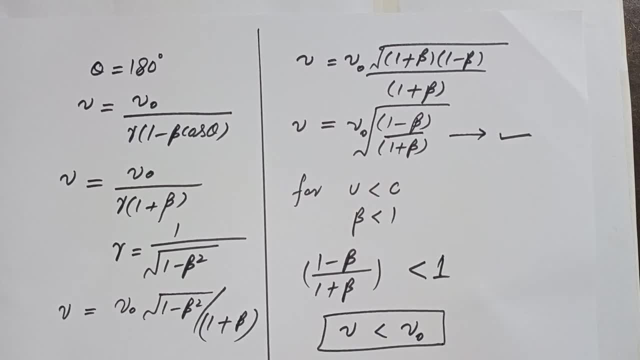 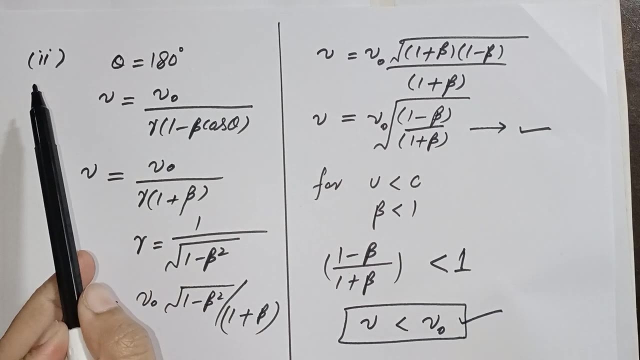 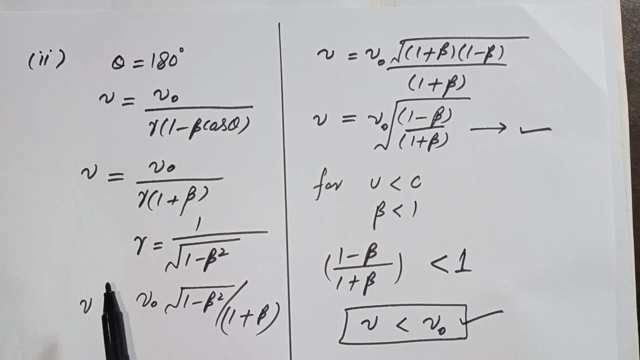 The observed frequency will appear to decrease as compared to actual frequency And it will be relative to caus sealing velocity of emitted light signal, which is nu, not. Next we will discuss a third case. like the source and observer move in perpendicular direction. 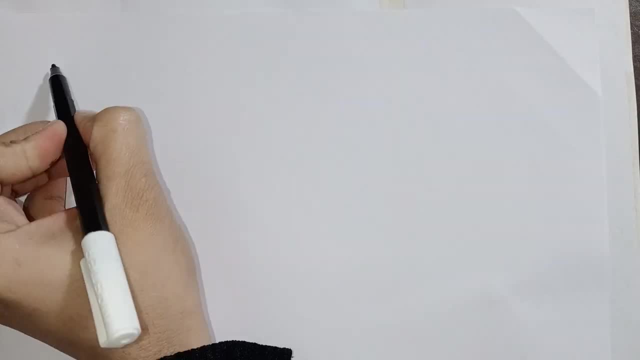 If the source and observer moves in perpendicular direction, then theta will be square into because it also moves in the sides. This will not change for v smaller than c, Because v isOf course having zero and the value of v smaller than length, which will die down. 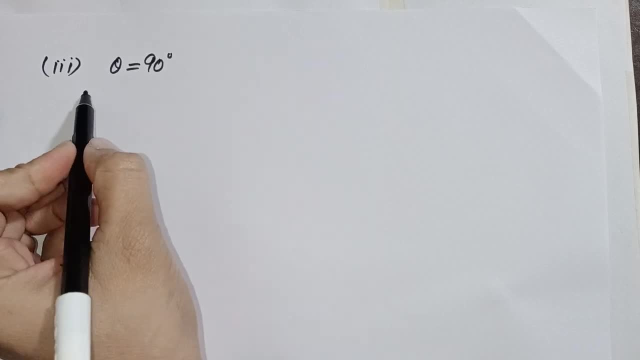 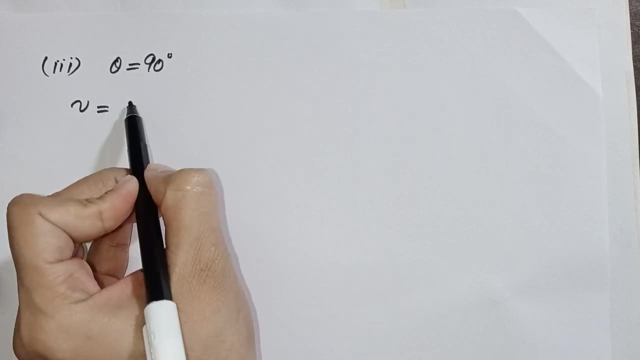 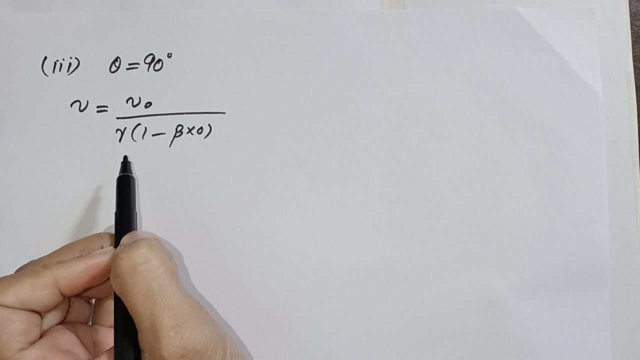 It will still differ between s recommendation and the second. comprehension 중 is also causing uh 90 degrees. now, substituting the value of cos 90, cos 90 will be 0 nu not over gamma into 1, minus beta into 0. nu will be equals to nu not over gamma. and using the value of gamma, 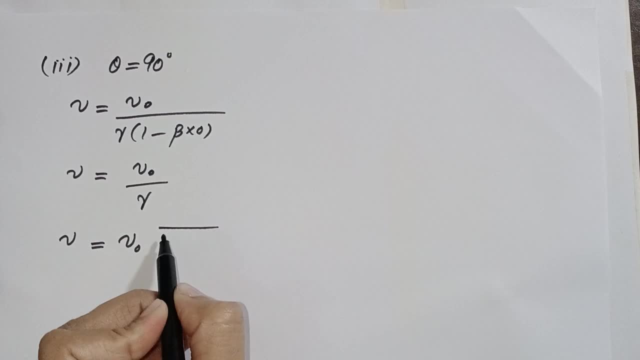 which is square root of 1 minus beta square. this is actually the value of 1 over gamma, square root of 1 minus beta square. Okay, beta square, since V is smaller than C for subluminal particles, again beta will be less than 1. for this value, beta will be smaller than 1. and if beta is smaller, 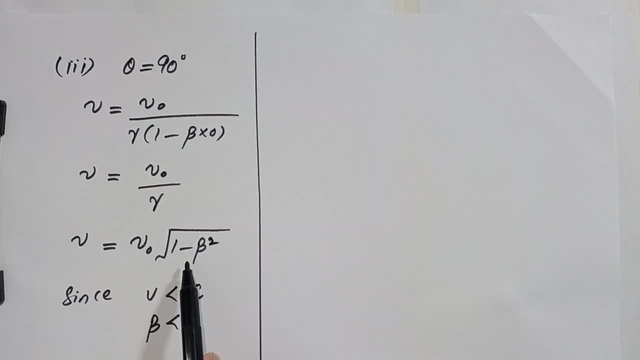 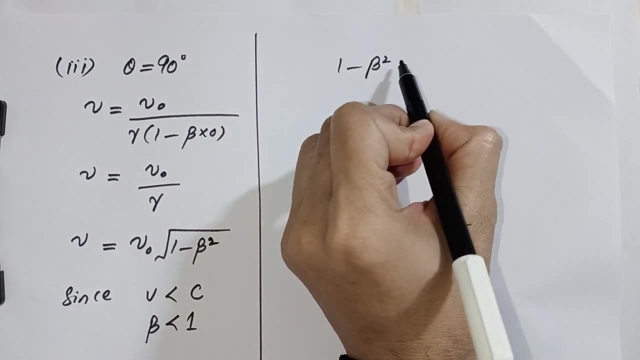 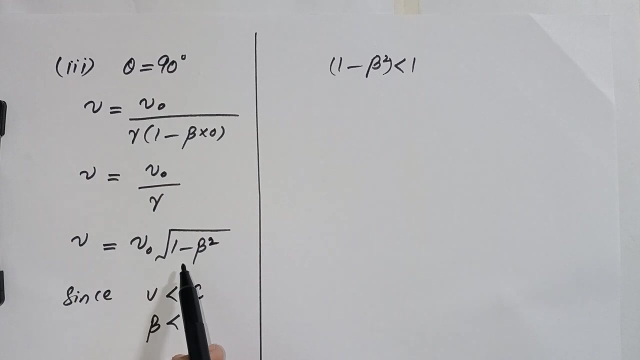 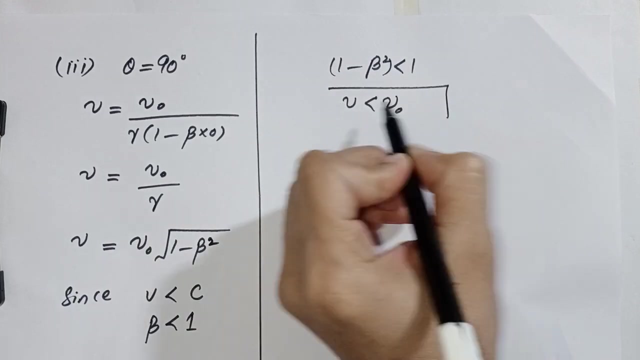 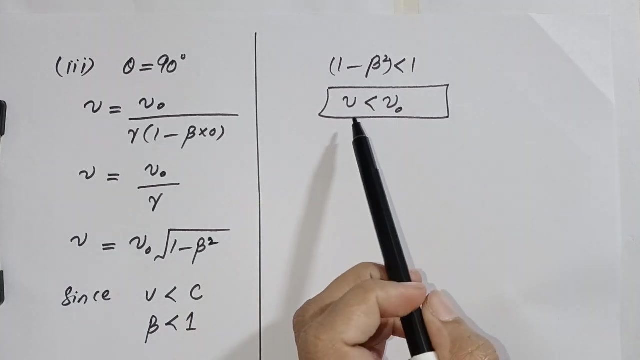 than 1, then this factor 1 minus beta square will be less than 1. 1 minus beta square will be less than 1, showing that nu will be smaller than nu naught. it means the observed frequency appears to decrease if the source and observer are in.